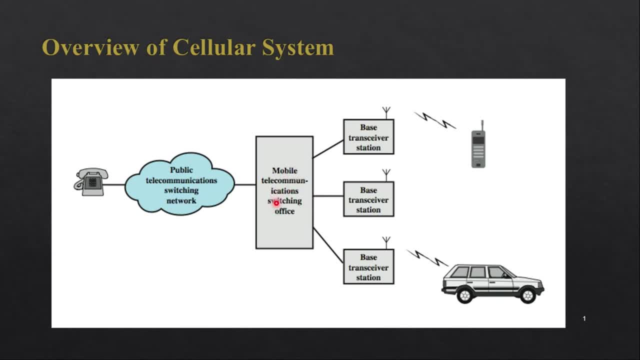 switching system. It is called as a mobile switching center or mobile telecommunication switching office. So whenever one user want to call a some another user, so it will be always gone through the BTS and BTS to MSC and again MSC to BTS of the another user. 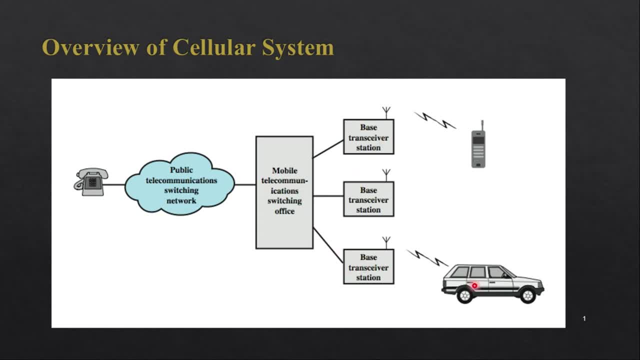 So this is how wireless communication is occurred in a cellular system. Now this MSC is also connected to other system like PSTN, public telecommunication switching network. So that is our telephone network. So if you want to call from telephone network to mobile user, so it will be go to the PSTN. 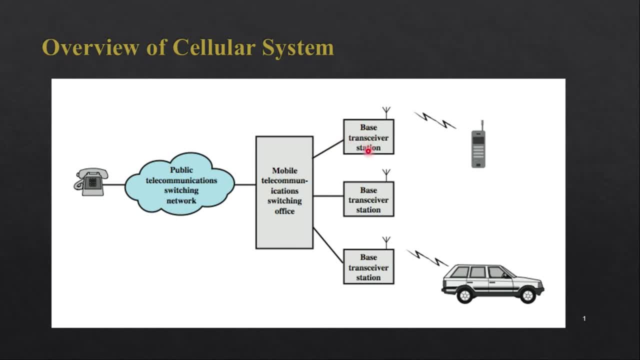 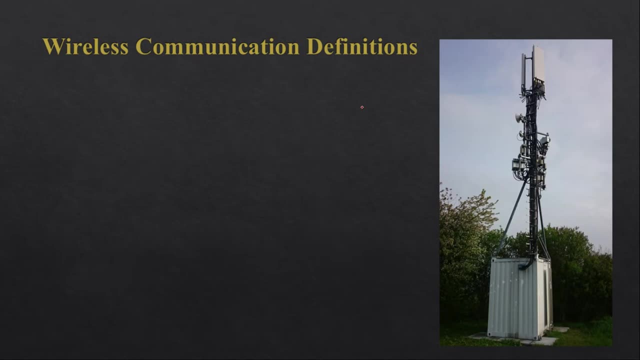 and PSTN to MSC and MSC to base station and base station to user. So this is how communication is occurred in the cellular system. So now we will. We will discuss the most important definition to understand the wireless communication subject. So first definition is base station. 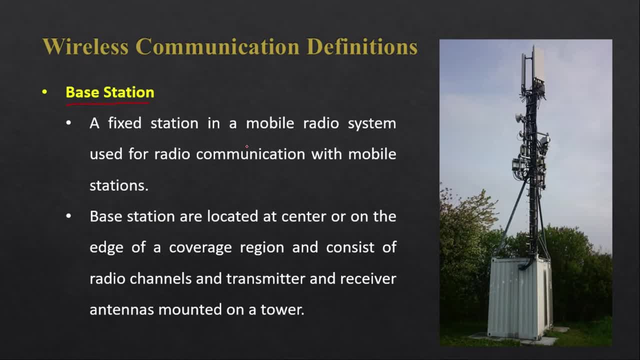 In a earlier slide I have told you that mobile station or cell phone is connected to base station. So what we mean by base station, Base station is a fixed station which is- you can see over here- This is the base station and it is a fixed station in a mobile radio system. 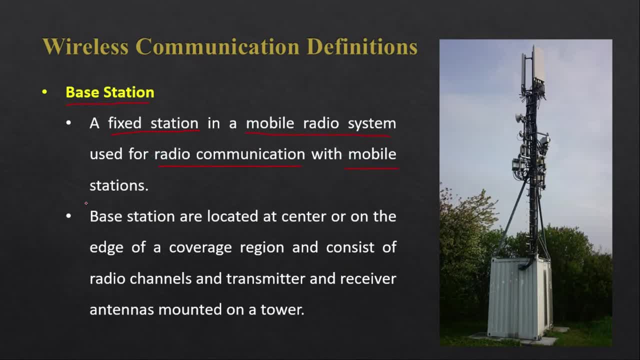 Use for radio communication with mobile station. So let's say, here we have one mobile, So this mobile will be connected to base station via radio communication And we will also discuss about the channels in the future. So this is the antenna that we are using to connect with the mobile station. 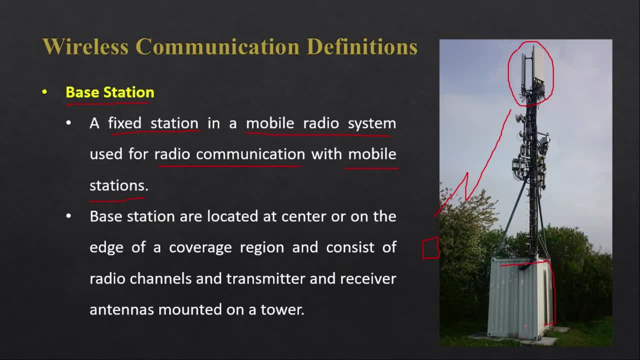 And this antenna is further connected to the BTS which will be over here. So this is the antenna, So this particular cell will have BTS battery backup and lots of thing, And here we have the feeder cable that will be connected to the BTS. 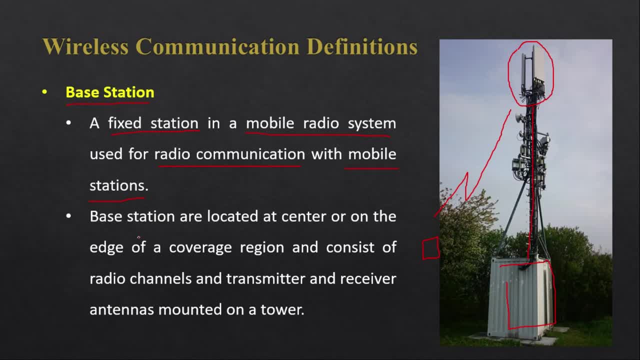 So all the switching operation is done by this BTS. So base station are located at the center or on the edge of the coverage region and consists of radio channel transmitter and receiver antenna mounted on a tower So that antenna You can see over here. and this is just a overview of base station. 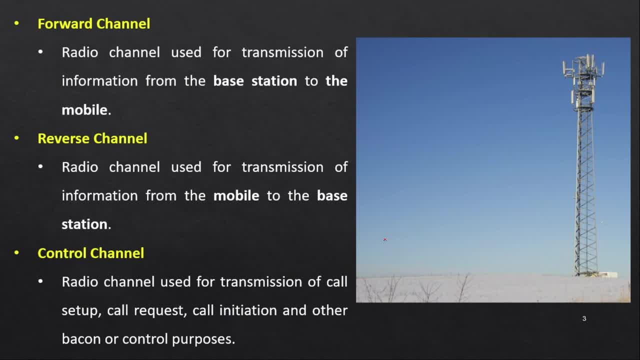 Next, we have a different kind of channel that is present in a wireless communication. Now, to understand this concept of forward channel, reverse channel or control channel, Let us consider that this is our base station and here we have, let's say, mobile phone, And first let's talk about forward channel. 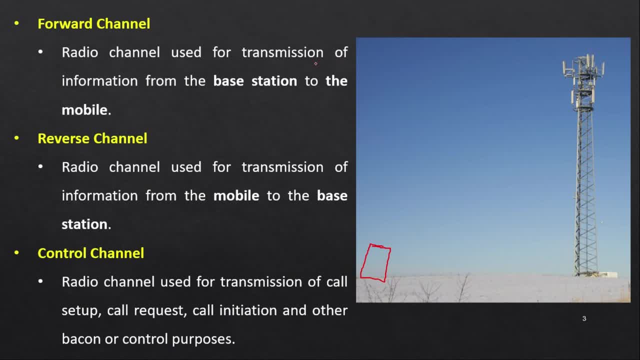 So forward channel is a radio channel Use for transmission of information from base station to the mobile station. So any information that is coming from this base station to this mobile station is known as a forward channel. It is also called as a downlink. 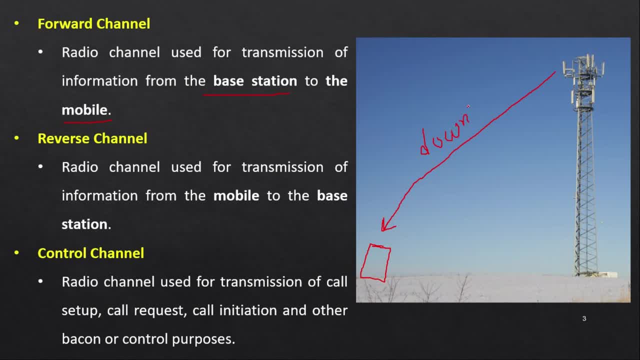 So, let's say, called it as downlink And it is from base station to the mobile station. So this is the downlink And this is the forward channel. Remember that this is not a physical channel. We are just allocating a frequency for communication purpose and this is a logical channel. 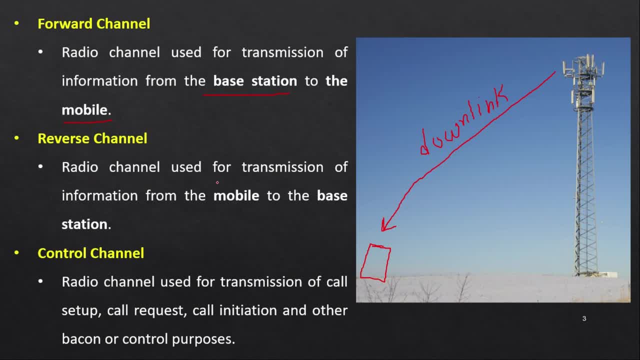 Similarly we will have a reverse channel, Radio channel used for transmission of information from mobile to base station. So during the communication, mobile station will also send information to base station. So that is what we call as a downlink And it is also called as uplink or reverse channel. 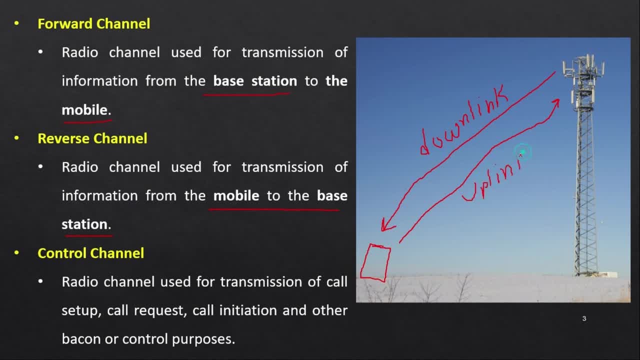 So any information that is going from this mobile station to this base station is called as a reverse channel or uplink, And we have a control channel. So it is a radio channel used for transmission of call, setup, call, request, call initialization and other beacon or control purposes. 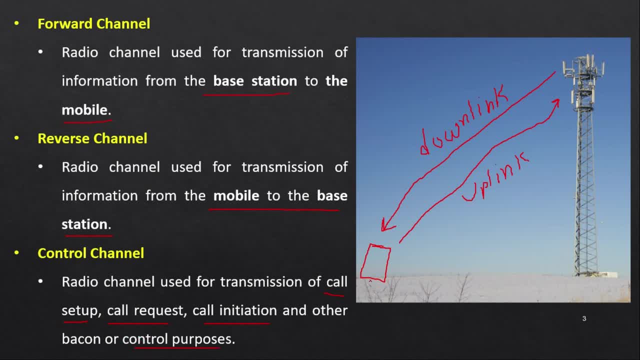 So with the mobile phone we have a control channel. So it is a radio channel used for transmission of call setup, call request, call initialization, call initialization and other beacon or control purposes. With the mobile phone we are calling someone, we are requesting or we are receiving the. 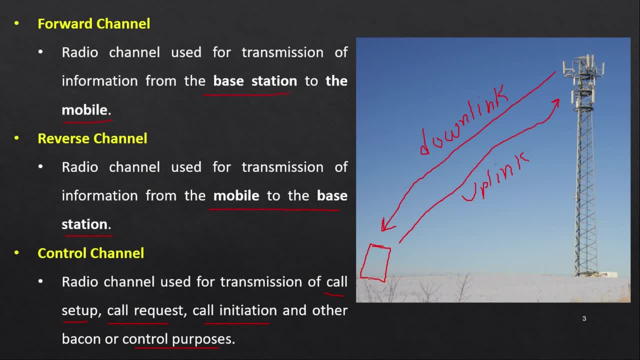 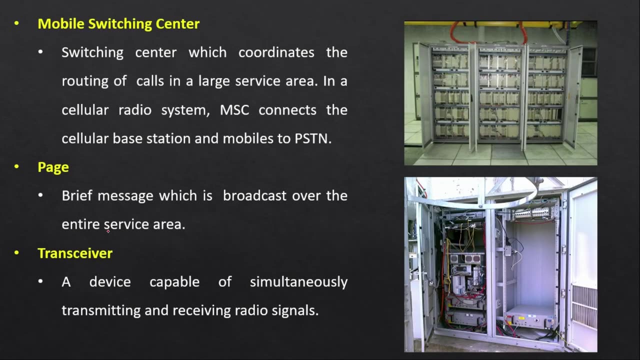 call. So for all this process, all this control process, we are using a control channel in the cellular system. There are other radio channels are also there that we will discuss when I will discuss GSM standard. Next, we have three more definition, that is, mobile switching, center page and transceiver. 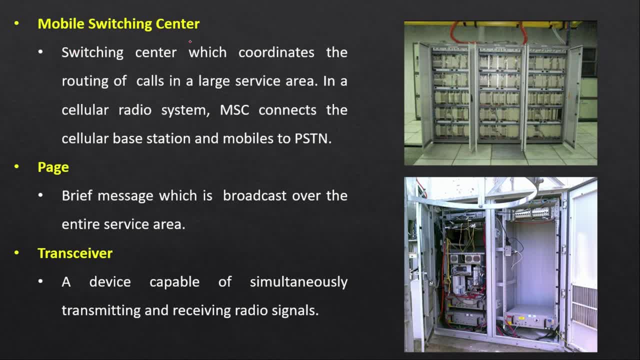 So first we have a mobile switch center, So this is a mobile switch center. First let's discuss about mobile switching center. So here you can see that it is basically a switching center, So switching center which coordinate the routing of call in a large service area. 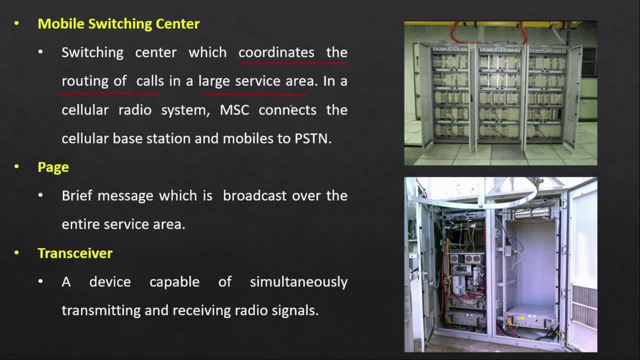 The function of MSC- mobile switching center is also called as MSC- is to communicate with the base station as well as some other kind of system, for example PSTN or SS7. So in a cellular radio system, MSC connect the cellular base station and mobile to the. 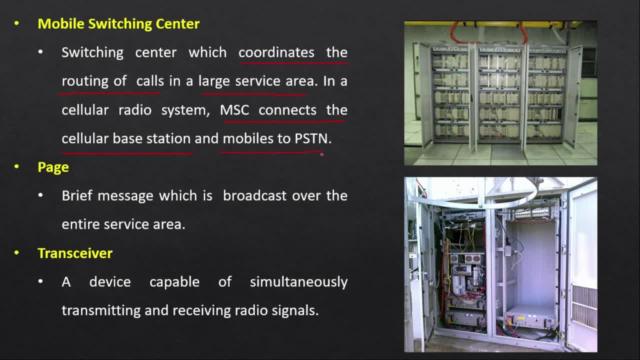 PSTN. So this is the main heart of the cellular system. Every communication will be done through the MSC and it will have a lots of register also that have a storage capability, and we will see these things also in detail. Next definition that we have is page. 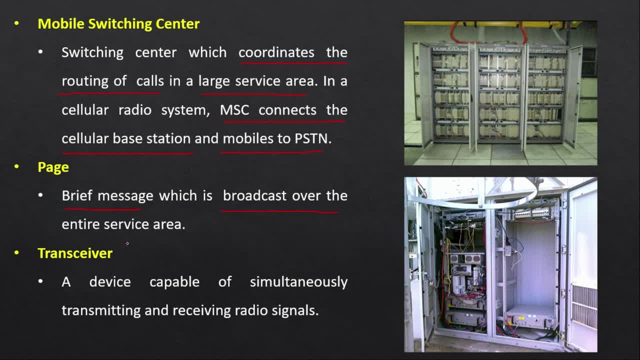 So page is basically a brief message. So this is a brief message Which is broadcast over the entire service area and it is sent by the base station to the number of users in a particular region. And last we have a transceiver. So transceiver is basically a device. in previous slide I have told you about BTS. that is base. 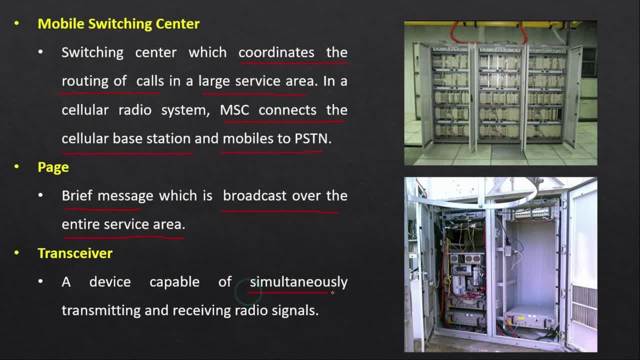 transceiver station. So it is a device capable of simultaneously transmitting and receiving radio signal. So this is how transceiver look like. So this is how transceiver look like And it has a capability of transmitting as well as receiving the signal simultaneously, and it has a lots of work at base station. 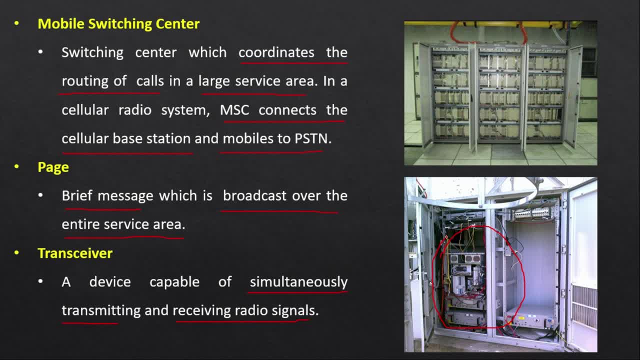 So these are the few basic definitions that you need to know to understand this subject. I hope this information are very helpful to you. There are many more lectures that I am going to upload for wireless communication lecture series. For that I need your support.